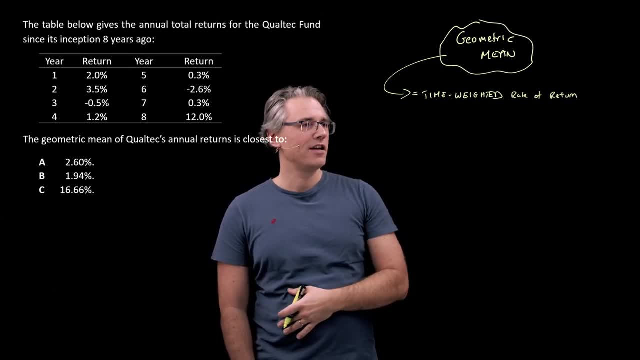 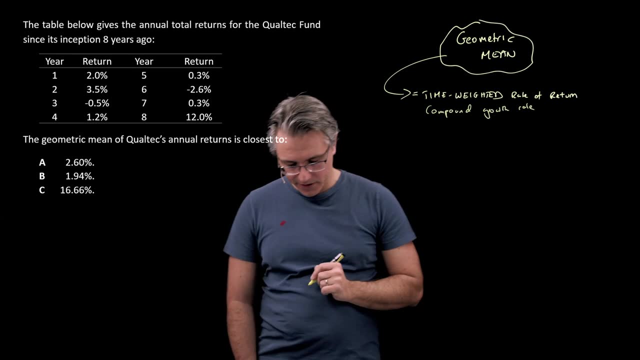 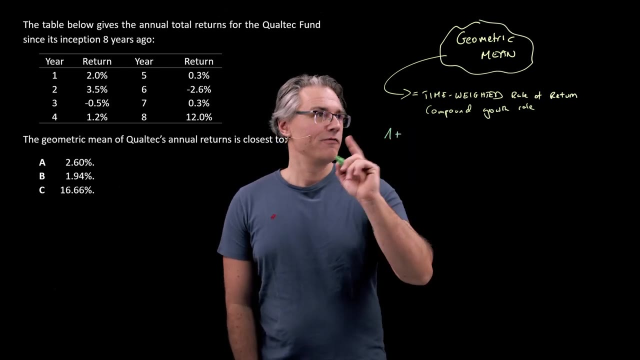 money weighted and time weighted rates of return. So time weighted rate of return or the compound growth rate? What do we mean by this? Well, in order to compute it, you're going to follow the following this logic: One plus of whatever is the geometric mean. I'm going to basically: 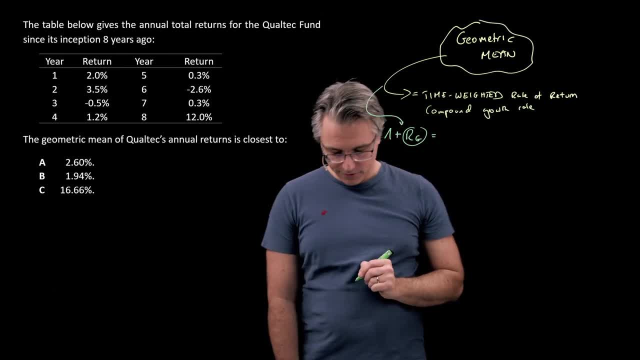 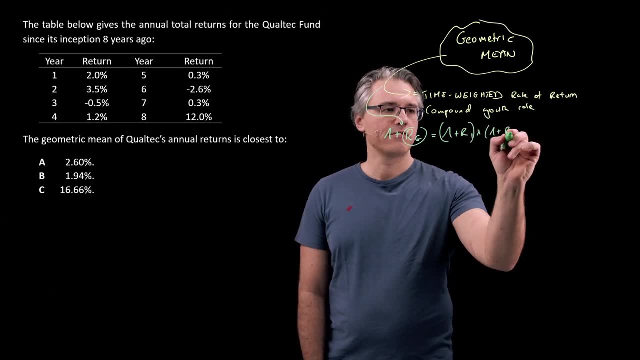 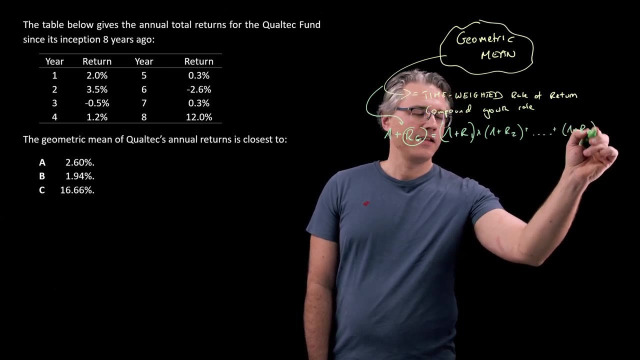 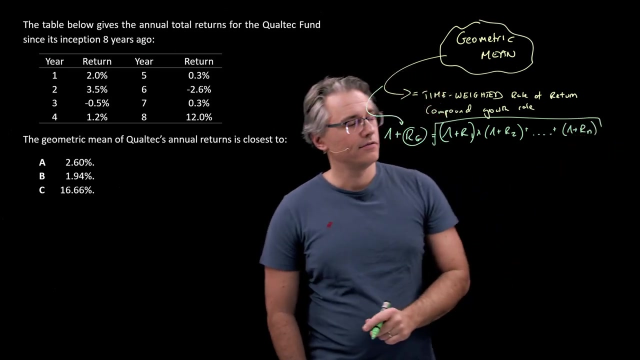 symbolize it as Rg is equal to one plus the rate of growth in the first period, times one plus the rate of growth in the second period. And you know this could continue for as long as there are periods ending with period n or the growth rate for period n, And you're going to have to take 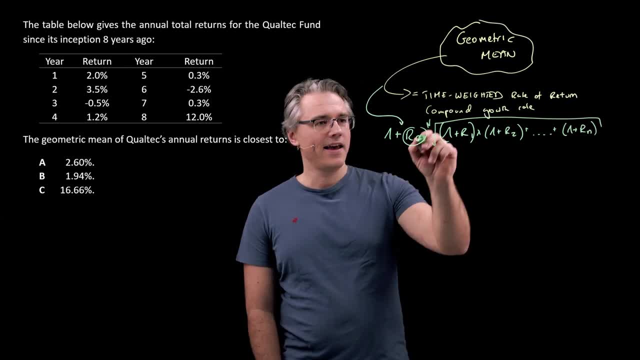 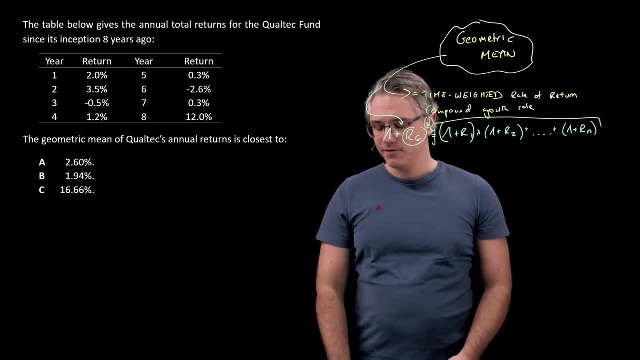 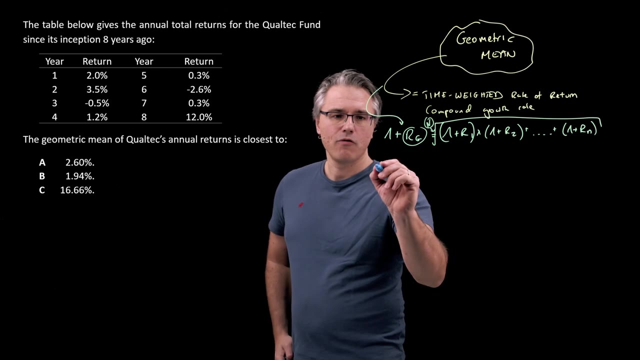 the root of the relevant exponent here, leave enough space for the n, so this n kind of belongs here and that's going to be your component: rate of growth. now, we're going to do this using the data in the question. so basically, if we type in the data, you're going to get one plus the rate of growth here, equal to- and let's 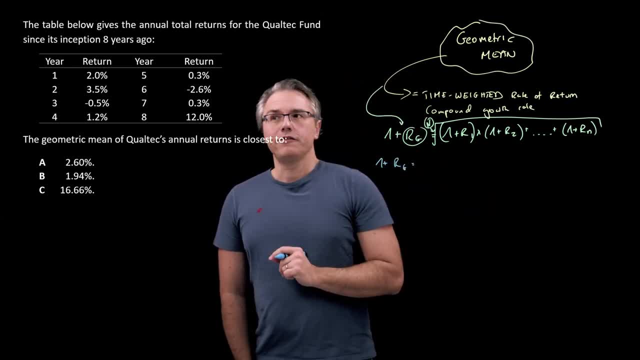 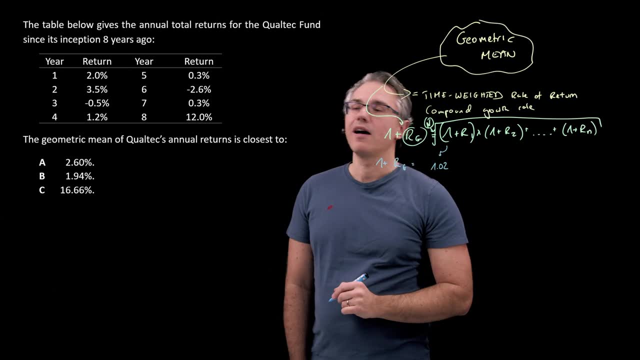 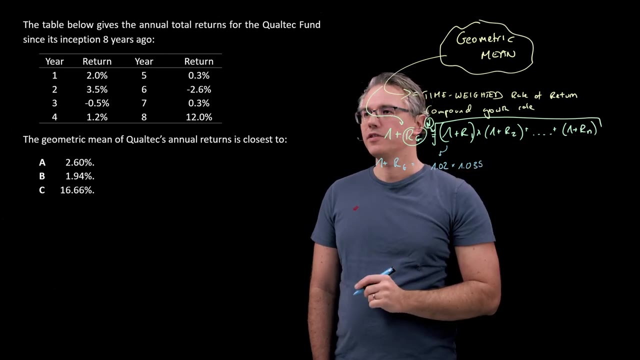 get the right numbers. for the first year it's two percent, so this is going to be 1.02. that's the same as saying 1 plus r1. now for the second year, we have 1.035, 1 plus three and a half percent. 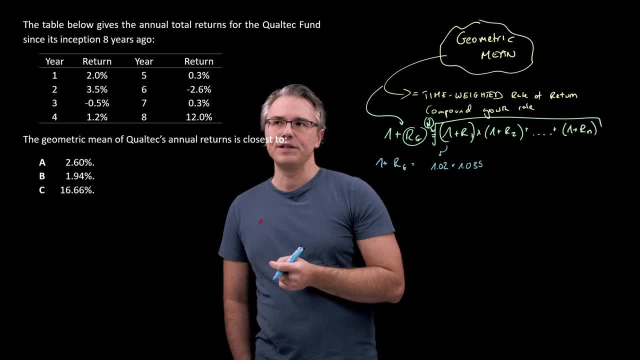 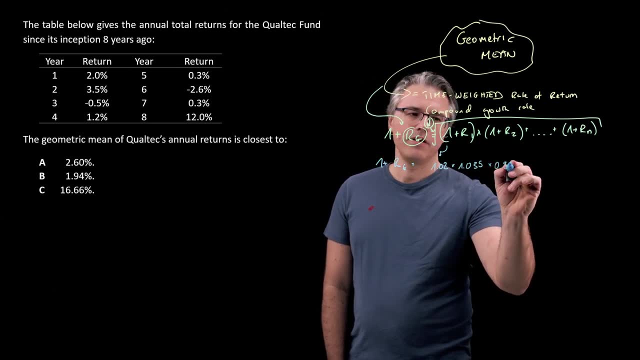 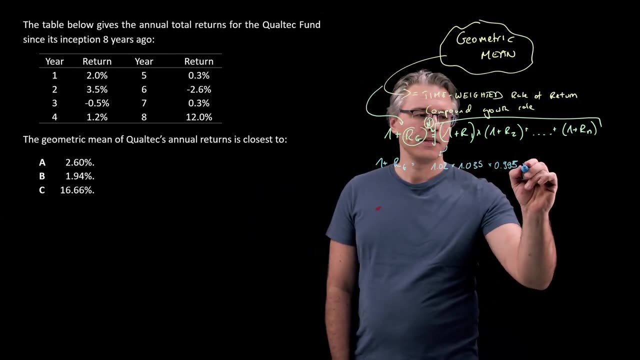 in this third year we've got a negative return, so it's going to be 1 minus 0.5, but that essentially equals 0.995, doesn't it? that's 1 minus half a percent. then easy, and this is actually where most people get wrong. they deduct the wrong. 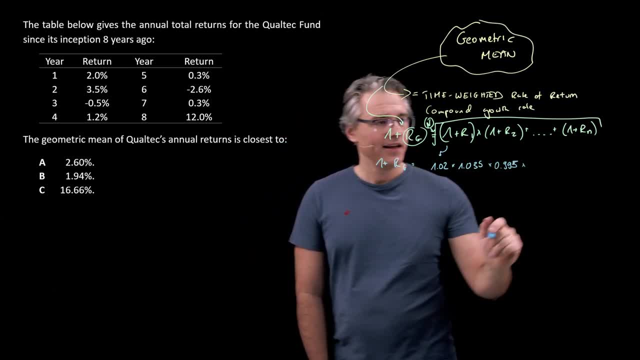 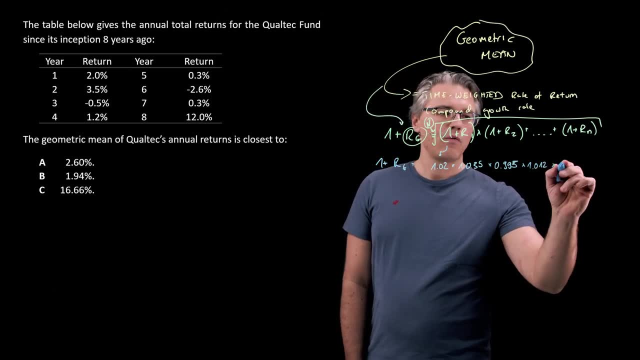 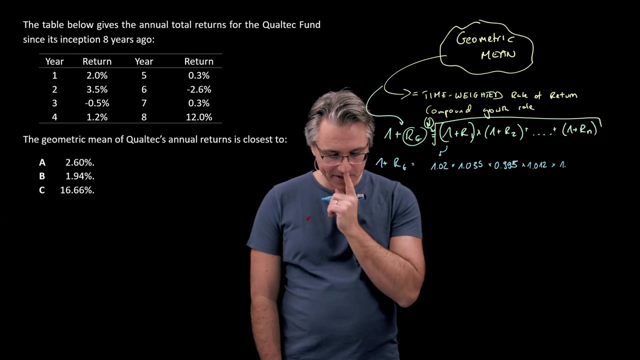 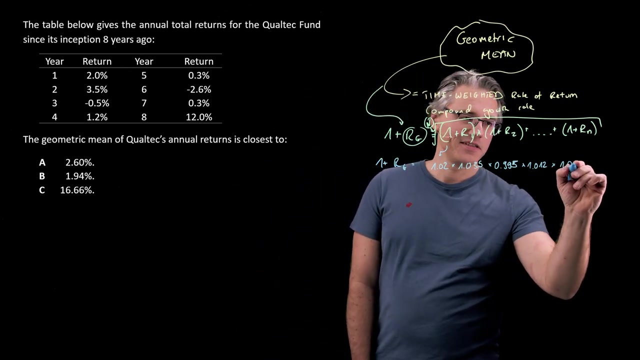 figure or they get stuck here. what do i do when it's negative? the next one is 1.012. now into the fifth year, one point and another place where you can get it wrong, getting the number of zeros wrong, because here it's obviously going to be 1.003, not 1.03. so this is another place where you can. 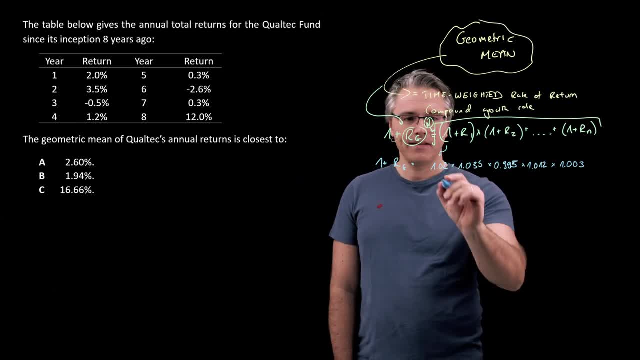 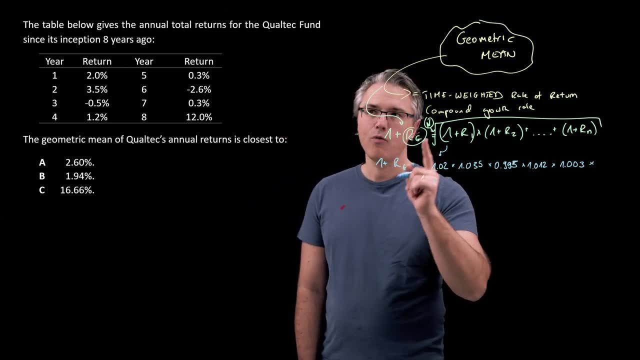 get a very easy mistake to make and then, uh, yeah, let's move over. here we've got a negative 2.6, so once again, think about what this would be. 1 minus 2.6 is 0.974, obviously, if in the exam you're a. 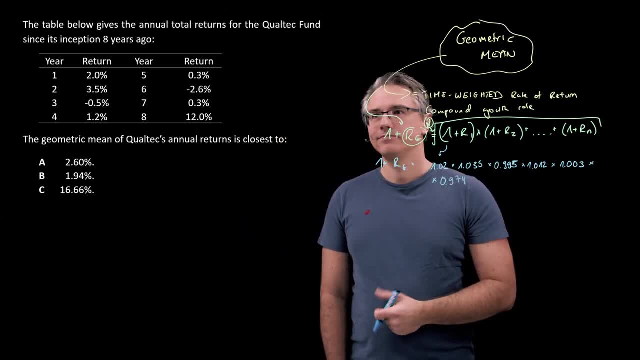 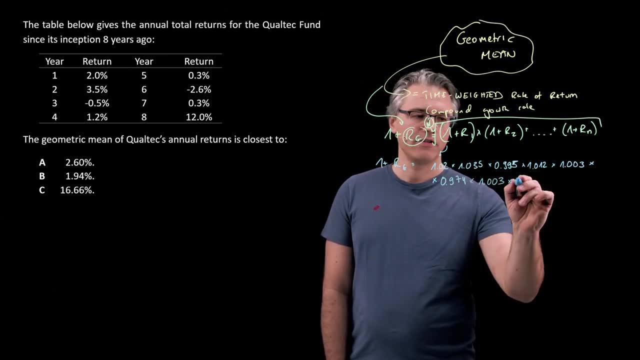 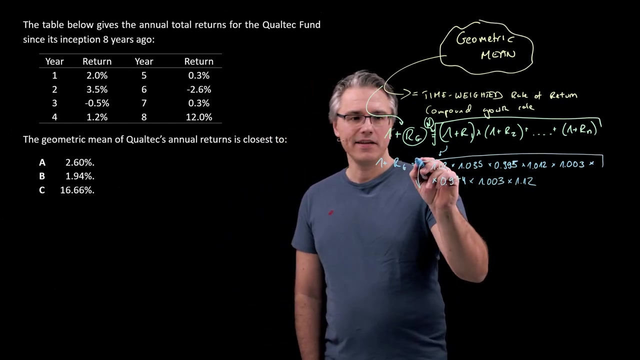 little bit stressed about getting this wrong. uh, potentially. um, just do it on the calculator. so we're going to do 0.003 again and we've got a 1.12. good, we're supposed to do all this and take the relevant um, you know, um a root and that's going to be the root of 8. 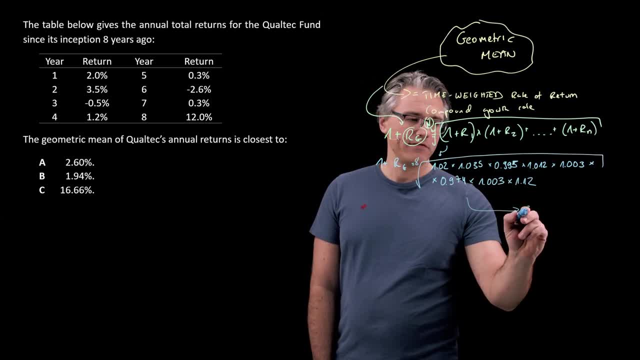 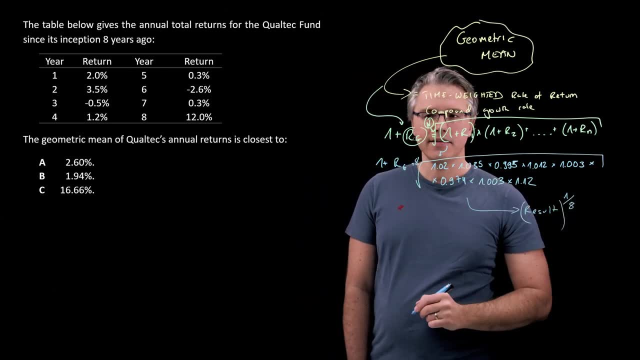 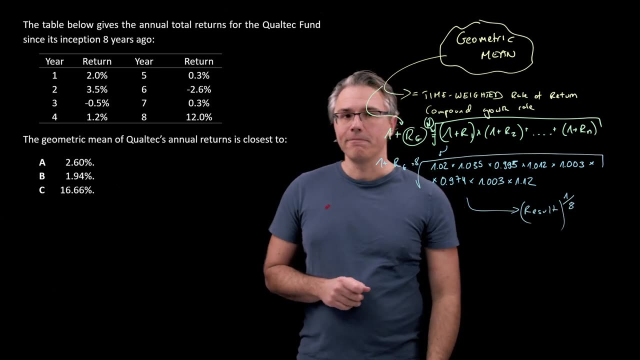 but this is the same as saying: whatever is the result here, we raise it to a power of 1 over 8 and obviously we deduct 1 to get the relevant result. okay, just the, just the r. so let's do this on the calculator, let me. 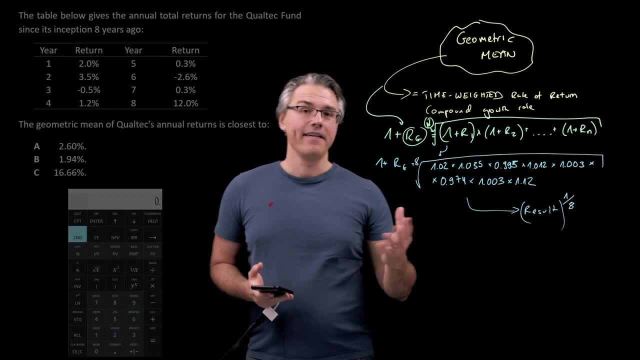 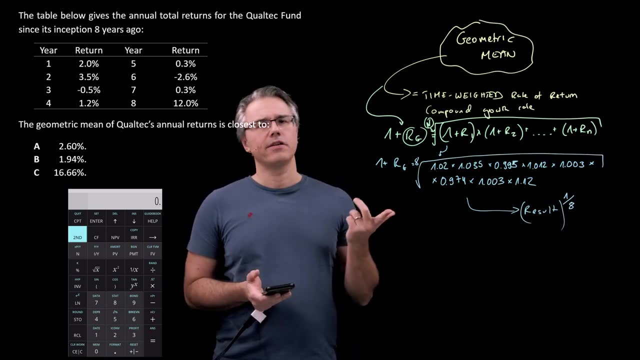 show you my calculator display. okay, so, assuming your calculators are set up properly using aos algebraic operating system, this shouldn't really be a problem. however, even if they're not, this should still work, i guess, because there's a lot of multiplication involved. let's do it. 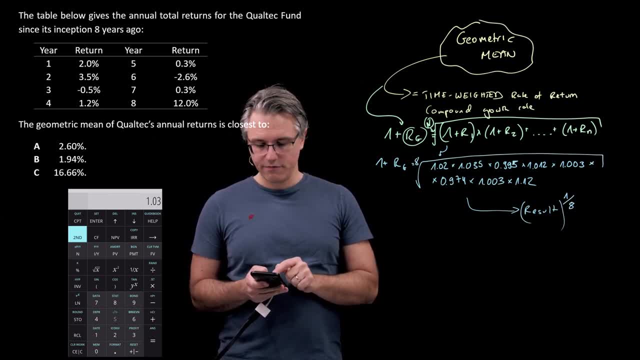 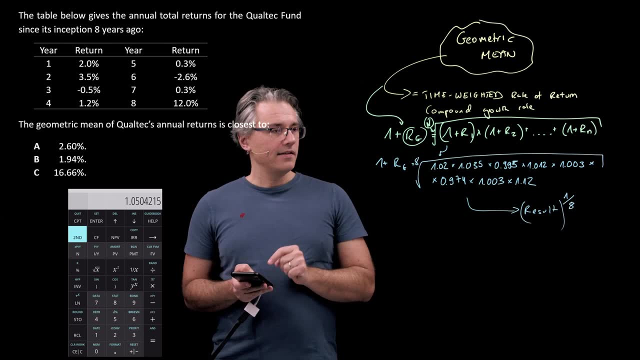 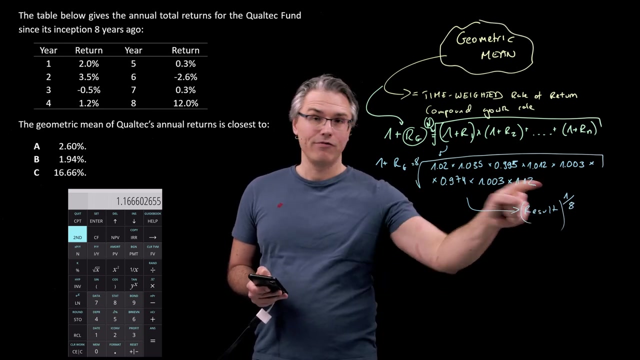 1.02 times 1.035 times 0.995- just be careful with what you enter- then 1.012 and times 1.003 times 0.974 and 1.003 times 1.12. okay, good, now you could go ahead and do the same with the other function. 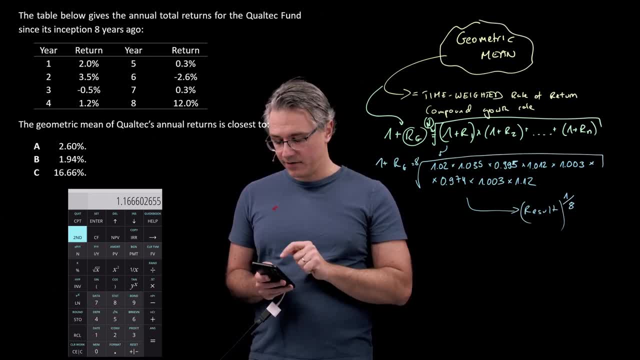 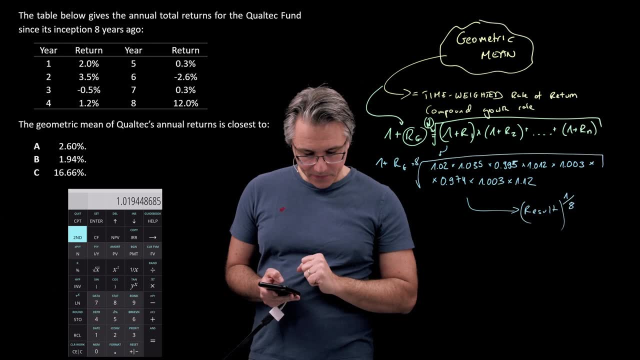 but you can raise this to the power of 1 over 8. so press the y to the power of x button. open bracket 1 divided by 8. close bracket equals: as you can see, i've got a result here, and this result reads 1.01944. now, in order to actually get the rg, which is the um geometric mean, i'm going to use the plus number on the right. so we're going to take a. 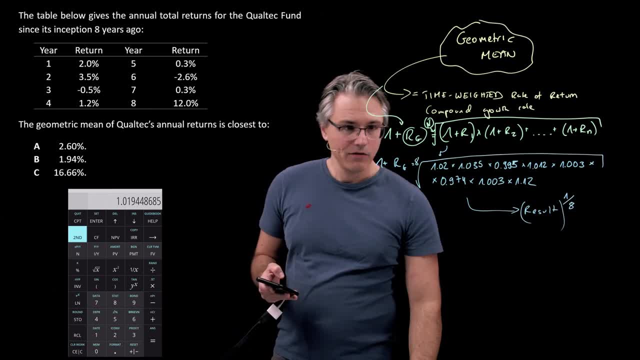 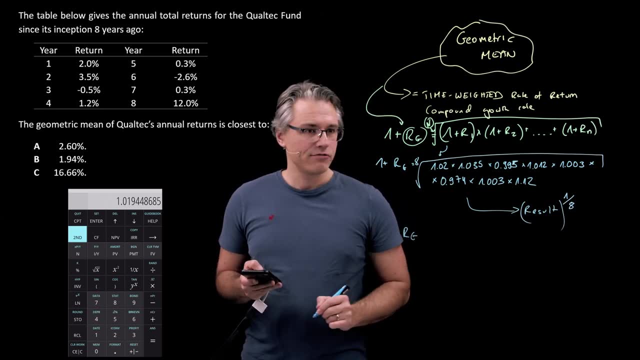 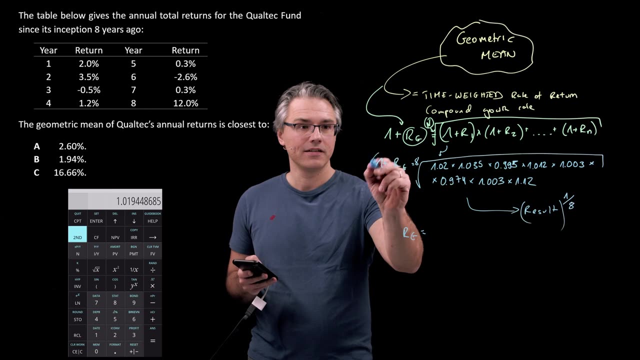 1.01944.. Now, in order to actually get the Rg, which is the geometric mean, I'm going to take this 1.01944 and deduct the 1, because whatever we computed here is 1 plus the rate. 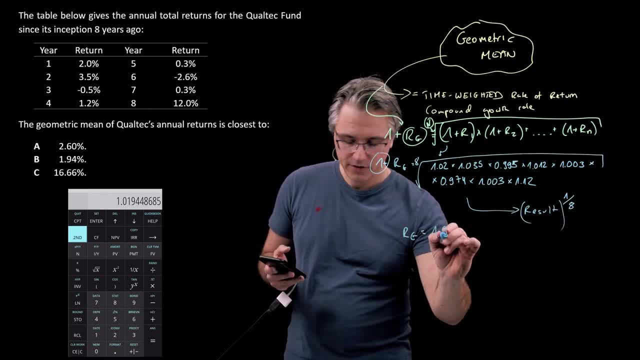 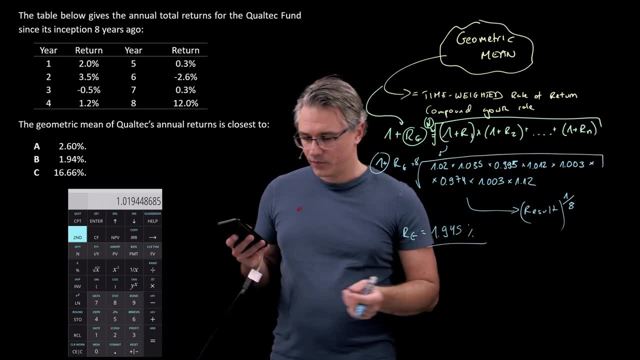 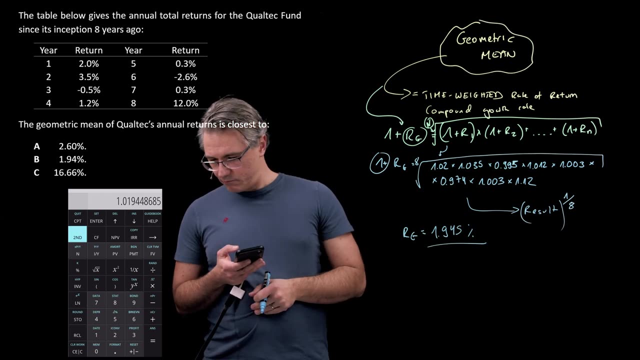 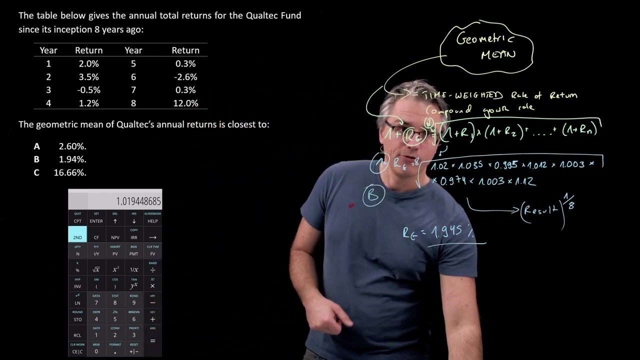 So ultimately, this ends up being 1.945, more or less percent, And that is the geometric mean in this question, which absolutely corresponds with what we've got provided as answer B. Now what does this geometric mean stand for and why is it so useful? Well, it shows you the 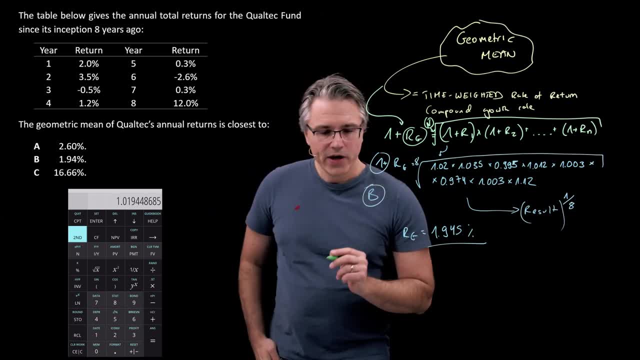 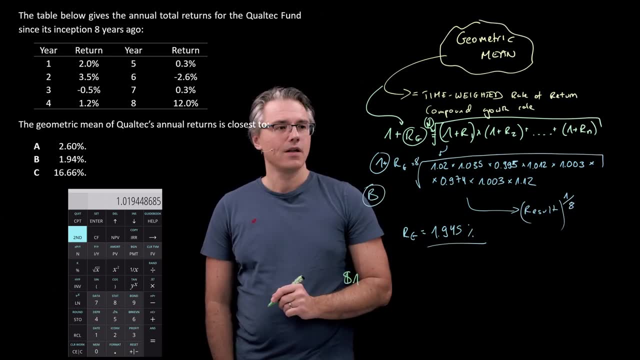 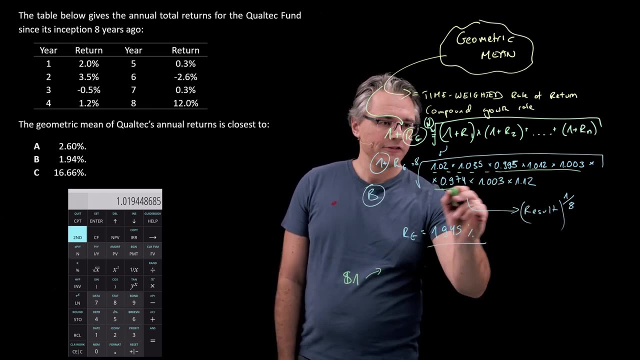 compound. It shows you the rate of growth. So if you had a symbolic 1 pound, 1 dollar, 1 euro invested into the fund, it would over time grow by these factors every year, either going up or going. 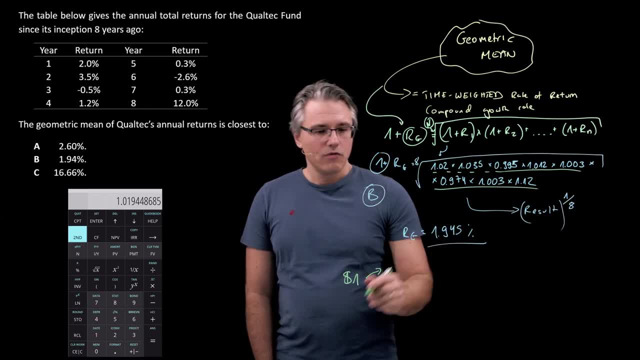 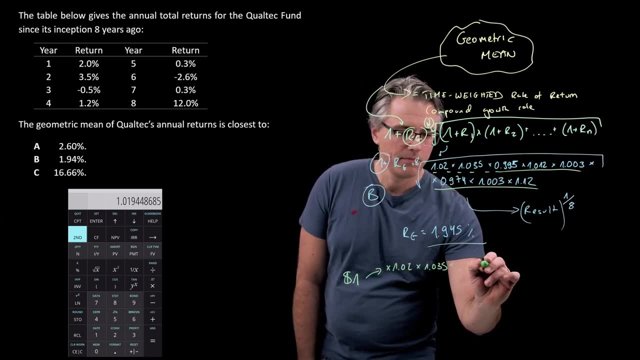 down depending on the fund performance. So you know times 1.02, times, 1.035, times. you know, and I'm saying that in the end you would, in the final year, have times 1.12,. 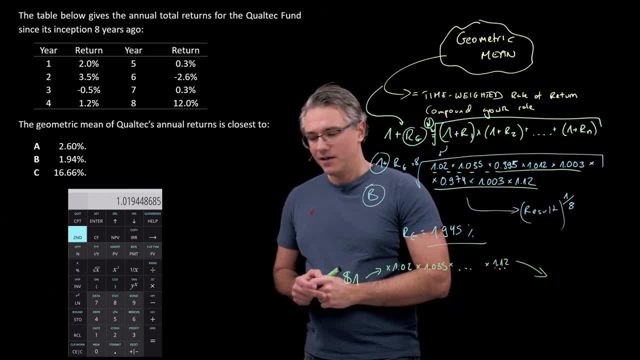 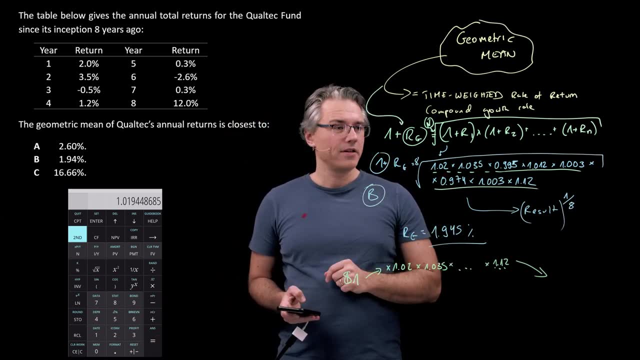 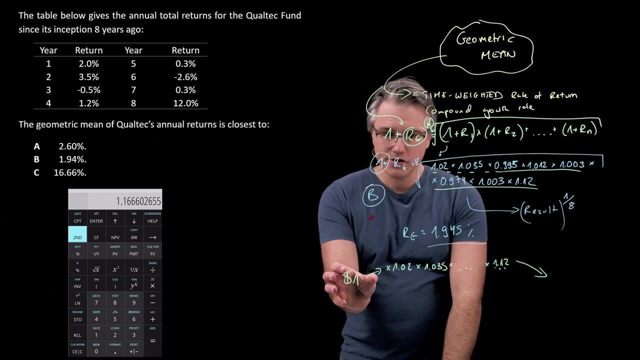 wouldn't you, And you would get to a certain result. And previously, when I was computing this, I had this result over here and I could now replicate it because I could raise this to the power of 8 and see what it was. Well, my 1 dollar invested initially at time 0, after 8 years of 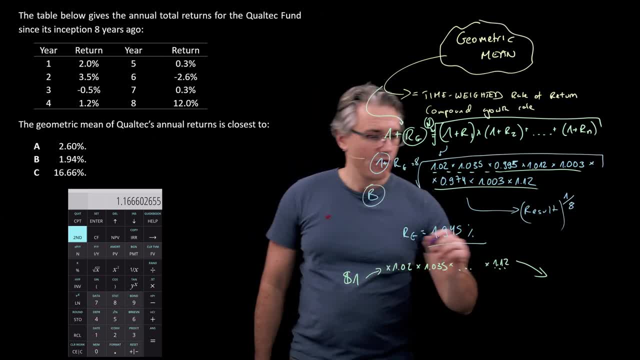 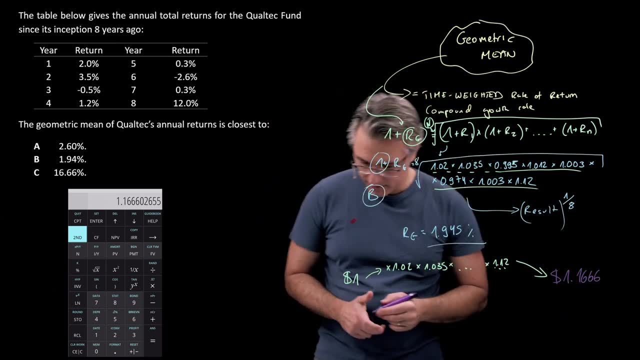 such growth would end up being 1.0.. So you know I'm saying that in the end you would, in the first year, be worth 1 dollar and 16.66.. Okay, That's the result I see on my calculator. Good,